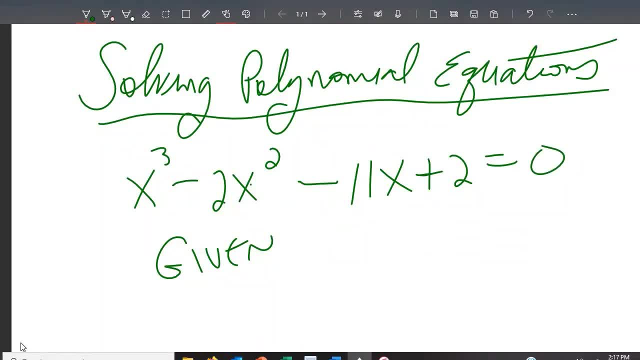 Let's say I want to solve this equation and I'm. We were given that negative 3 is a root. Now, remember the word root also means zero and we use synthetic division to help us solve this. Let me do this one more time, just to make sure you remember. 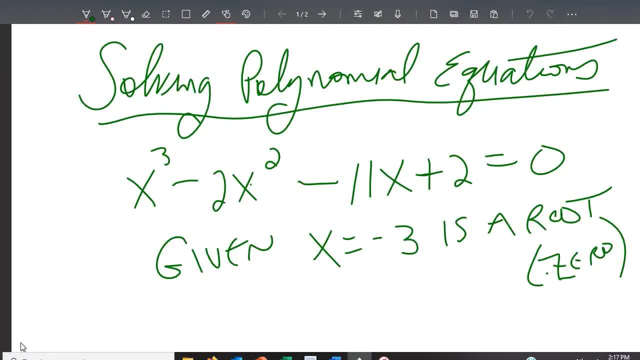 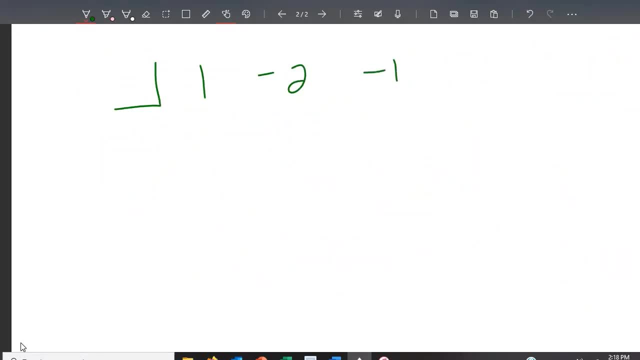 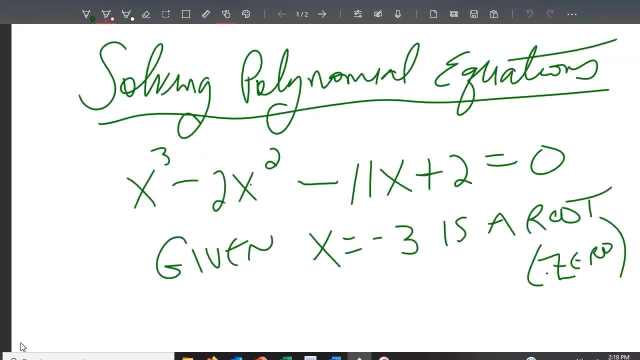 All right, so we bring down the coefficients, So it's going to be 1, negative 2, negative 11, and 2.. The number that goes here- remember when it gives me this information, when it's written like this- that's the number that goes in the little half box. 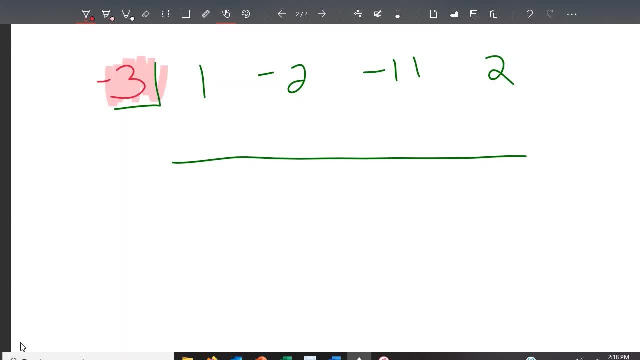 It's giving me the number to put in here already. Now. let's do the synthetic: Bring down the 1.. Now, since I'm told it's a root, I should get a zero right here. If I don't get a zero, then this book is wrong. 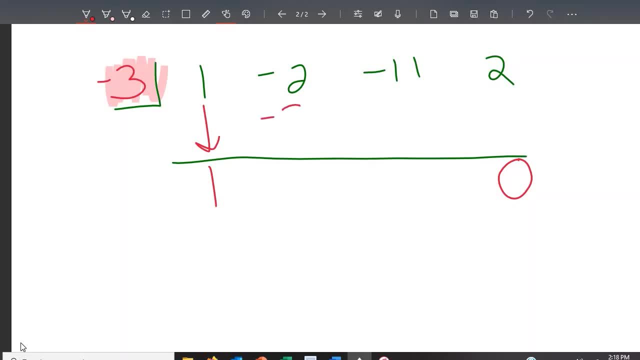 So there we go. So multiply Negative 3 times 1 is negative 3. Add the two numbers Negative 1, negative 5 times negative, 3 is positive 15. I get 4.. Hold on, I must have wrote. 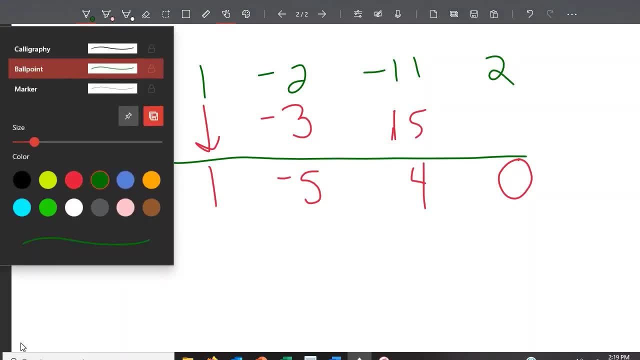 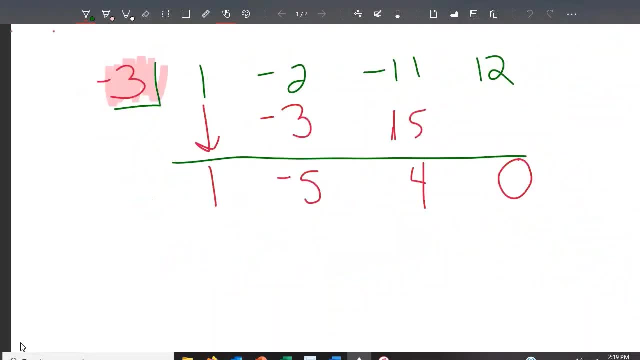 This should be a 12, not a 2.. I wrote it down wrong. That's a 12 right there. Okay, so 4 times negative 3 is negative 12. Which gives me My zero. So we bring down the numbers coefficients and put them back in front of the variable. 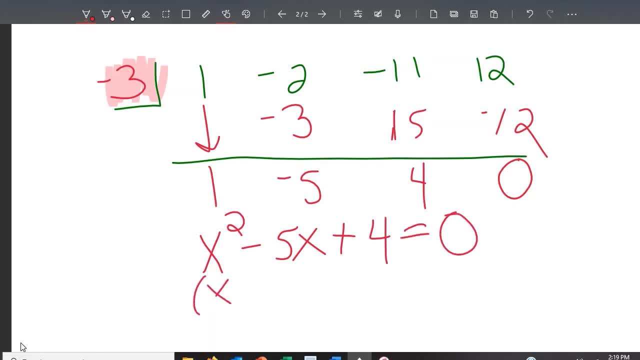 Set it equal to zero, Then we factor and solve for the other two roots or zeros or whatever you want to call them. So when we solve this, when x minus 4, we'll get x to be positive 4.. 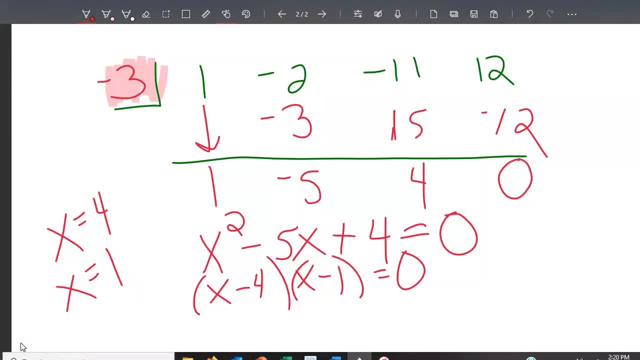 The x minus 1, x will be positive 9.. These are my three solutions, also called roots, also called zeros. Now, in this example, we were told what to put right here. Well, that's good. I need to know that in order to do these problems. 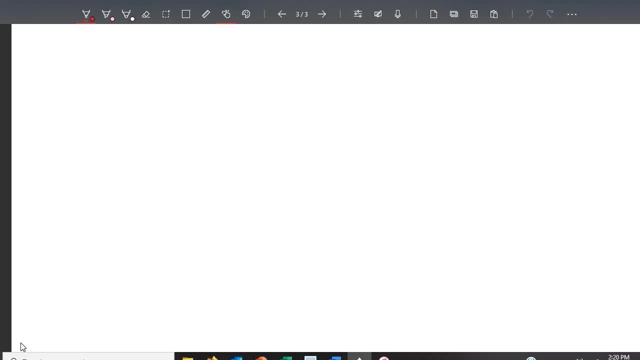 Now suppose, though, I gave you this: I said: solve x cubed minus 2x squared minus 7x plus No minus 4 equals zero, And that's all I tell you. Okay, I'm not told something. 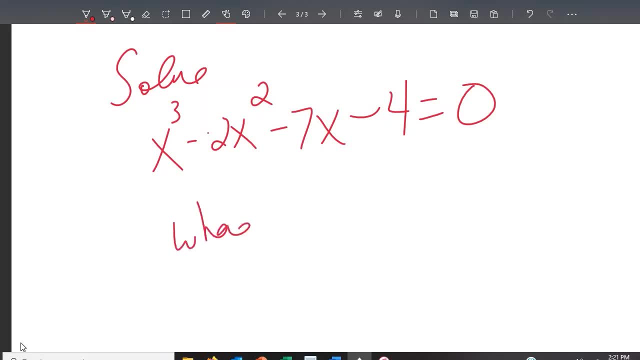 Well, where is a root? Where is the info about a root? Yeah, that's the problem in this section: We're not told what the root is. So what we have to do Is something called the Rational Zero Theorem. 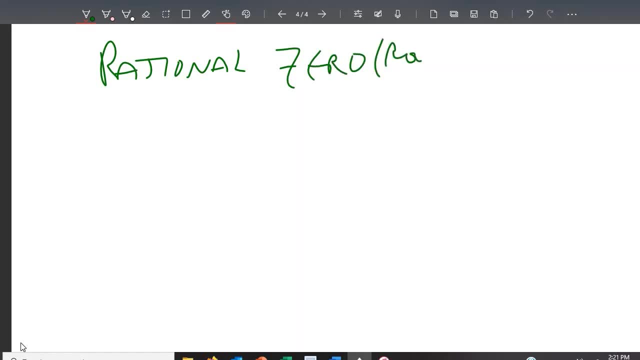 Or the Rational Root Theorem. What the Rational Root Theorem does? It creates A list Of POSSIBLE Roots And highlight that POSSIBLE. Now, this is POSSIBLE, That doesn't mean they are. It means this could be. 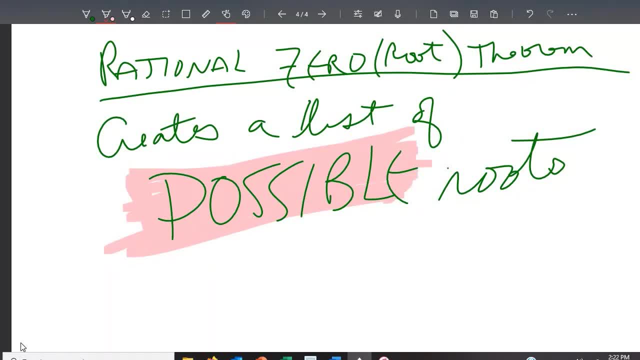 Now our lists are going to be. Some of them are going to be kind of long. I might have 16 POSSIBLE answers. I might have 4 POSSIBLE answers. I could have, you know, 30 POSSIBLE answers. 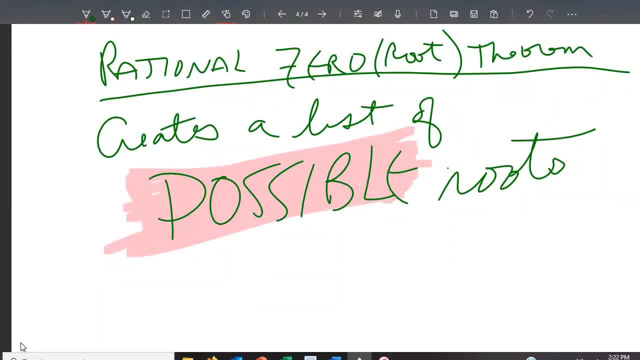 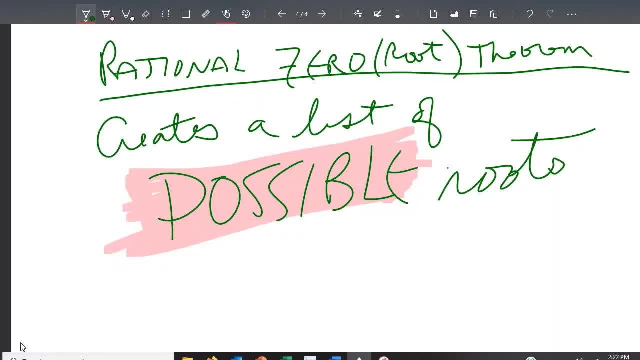 It's just tedious, And once we list this root, We're going to use Synthetic, Synthetic, Synthetic To find, To find A zero. So instead of us being told up front, We've got to go find it ourselves. 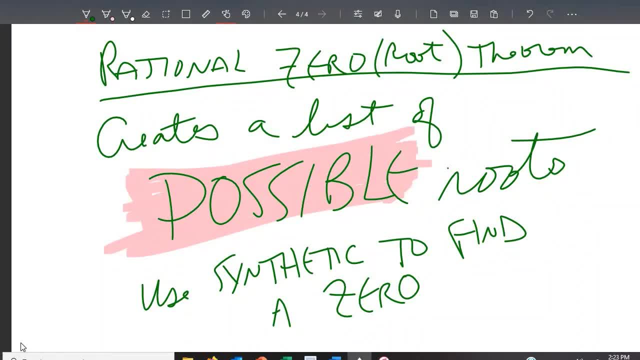 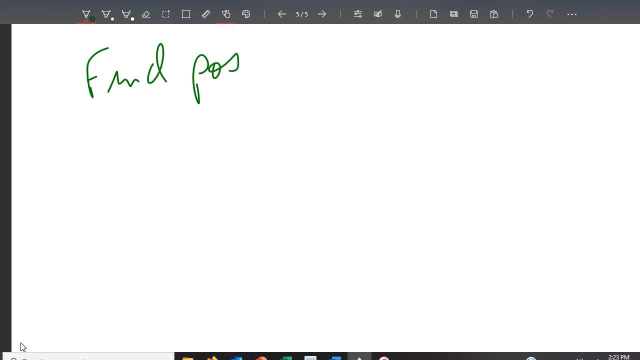 So, instead of us being told up front, We've got to go find it ourselves Now, In order to find the root. In order to find the root, Find POSSIBLE roots, Find POSSIBLE roots, Find POSSIBLE roots. What you do is: 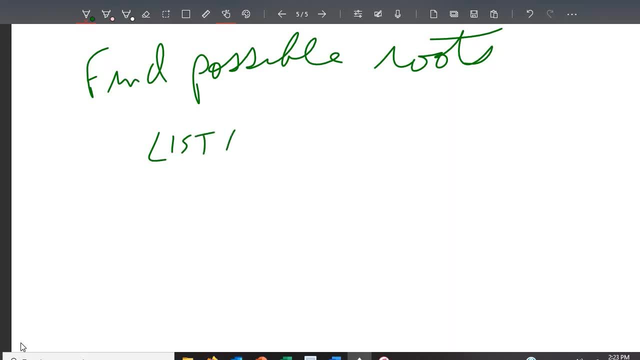 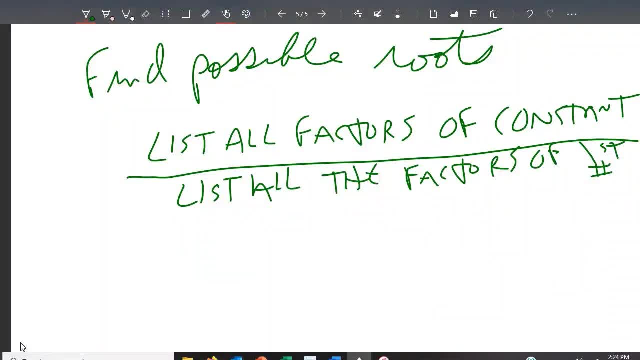 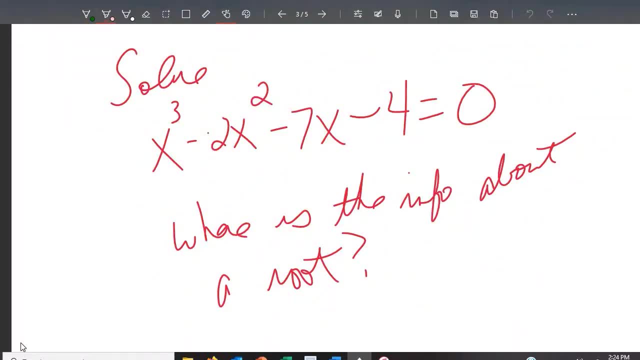 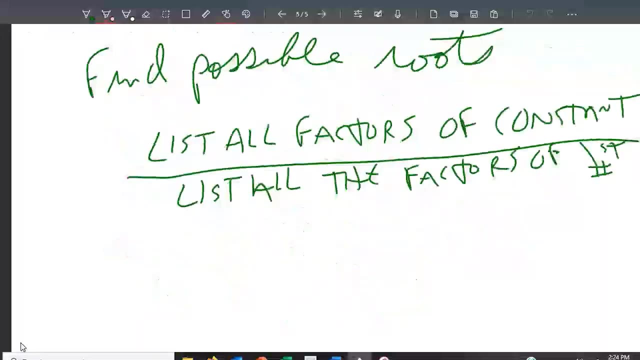 last number. now, what was this example I had over here? all right, so I want to take this one. now it's a four. this is gonna be a fairly simple one, so I want to list all the possible factors, I mean, find the possible roots for that previous example. so we're going to create a fraction when you're. 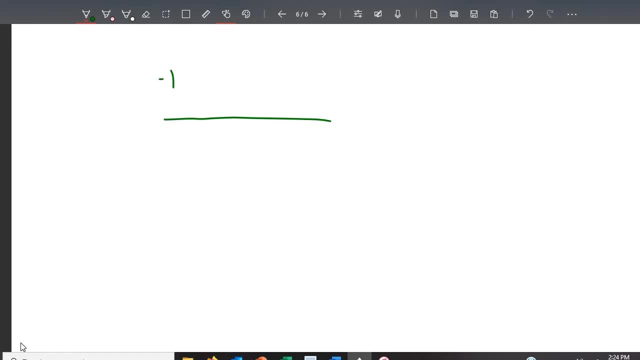 listing the factors. you must put a plus or minus in front of each factor, so factors of the last number go up top, the factors of the first number go in the bottom. you know, and it was just a plus, it was just a one. so that's good then. 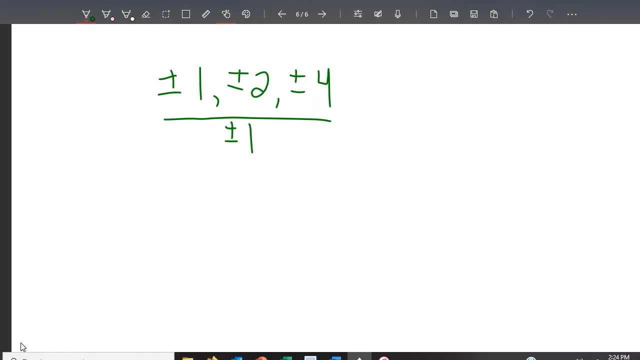 you take the each number in the bottom and you divide it by all the possible roots for that previous example. so you want to get it into each number in the top. in this case, we're just dividing them into when we divide them by one. so this is what we end up now. I want you to notice. 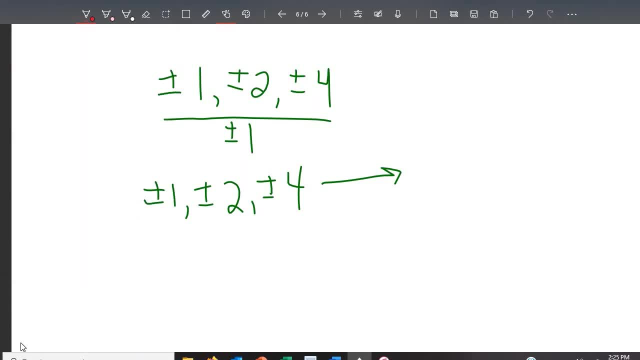 I have six possible roots. because of that, that plus or minus what I would do if I wanted to solve this equation. I would have to take each one separately, use synthetic division and then do this until I find a remainder of zero. but before I do that, I want to practice finding these possible groups. let's do. 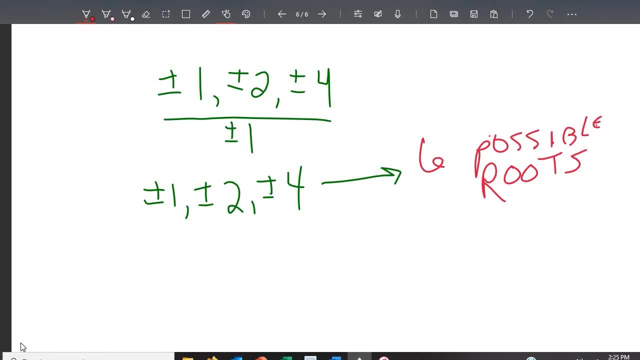 well, let's do this. let's um, let's say, I want to list all the possible roots. list all possible roots of 2x cubed or the function. this is a function: 2x cubed minus 3x squared minus 11x plus 6.. Now I'm only looking at the 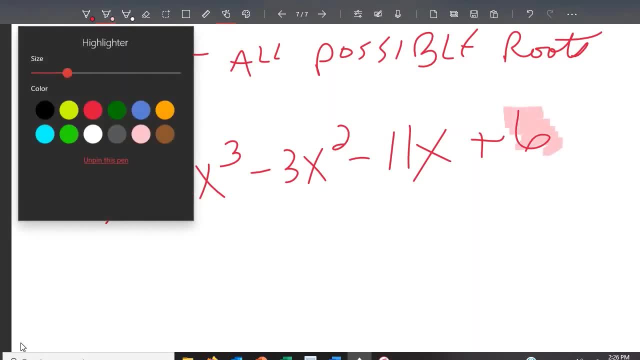 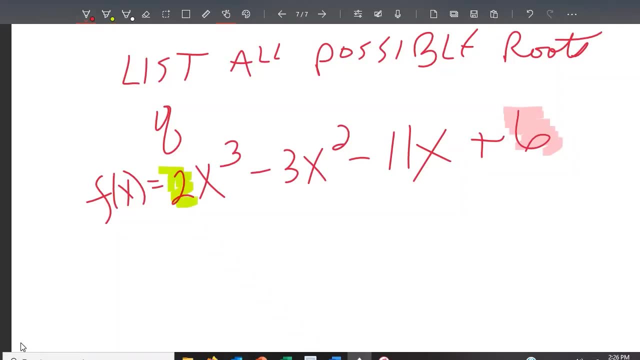 last number and the first number. I don't care anything about the negative 3 and the negative 11.. You've got to remember to put the factors of 6, the factors of the last number, over the factors of 2.. So it's the last number goes on top. 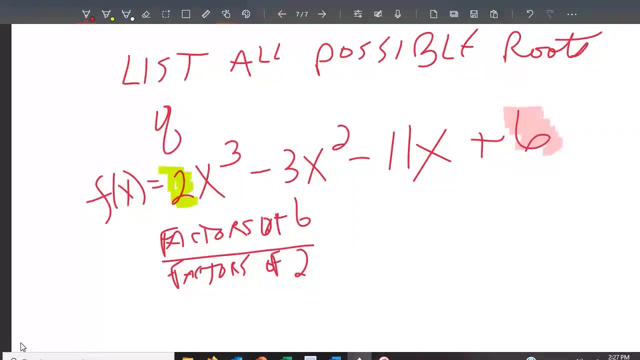 and the first number goes on the bottom. Now let's list all the factors of 6.. Now make sure you put plus or minus in front of each one. Plus or minus 2,. plus or minus 2.. Plus or minus 5.. Plus or minus 6.. Plus or minus 7.. Now, what am I doing? I'm listing. 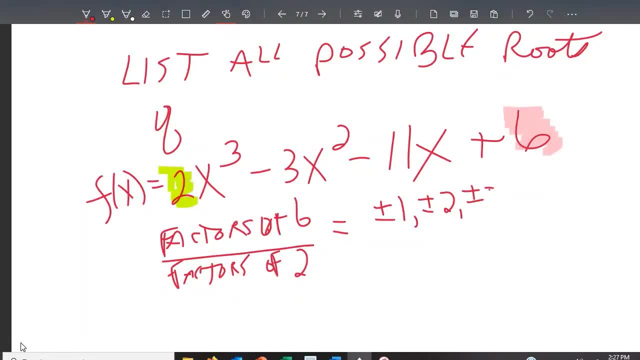 plus or minus three, plus or minus six. then you're gonna have in the bottom plus or minus one, plus or minus two. now here's where you got to pay attention. I'm gonna write it out the long way then we can simplify. you're gonna take each number in the top and divide it by each number. 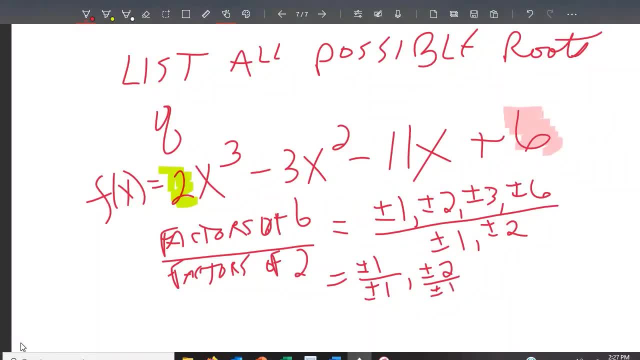 in the bottom separately. so it would look like this: which, all right, so that's doing the one. and you turn around and you'd say: okay, plus or minus one divided by plus or minus two. plus or minus two divided by plus or minus two. plus or minus three divided by plus or minus two. plus or minus six divided by plus or minus two. 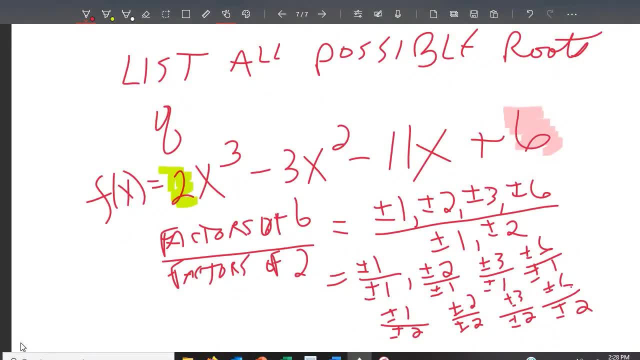 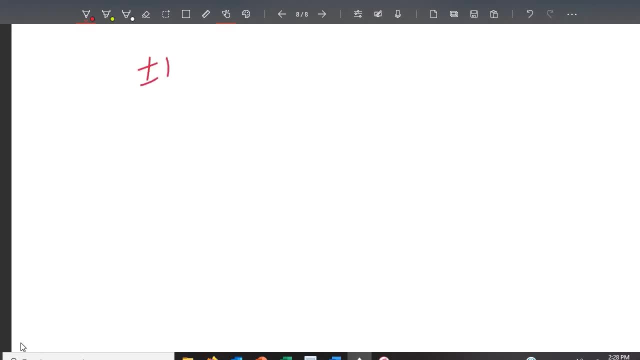 now you're going to go simplify these. I'm going to come over here to the next slide. so we're going to get: 1 divided by 1 is 1, 2 divided by 1, 3 divided by 1 and 4 divided by, I mean 4, 6. 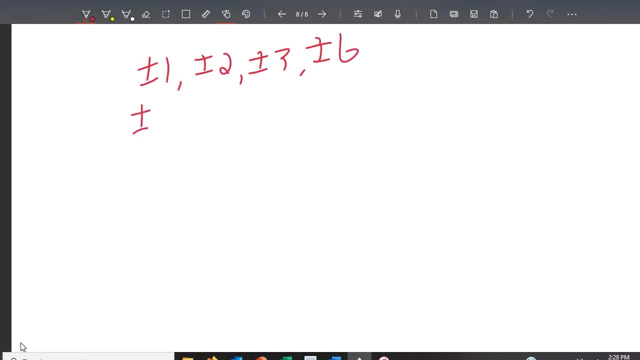 by 1, then we're going to have 1 divided by 2 is 1, half 2 divided by 2 is 1, which we already have. then we're going to have 3 divided by 2. then we're going to have 6 divided by 2, which is 3. 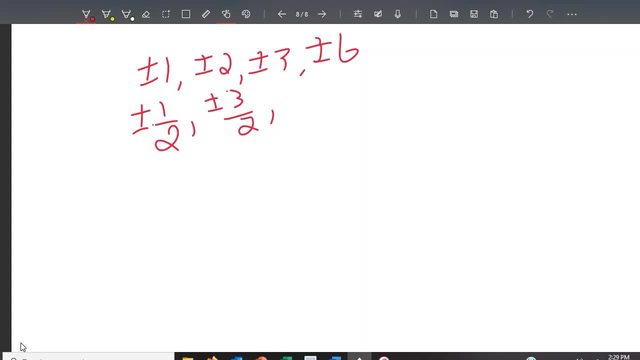 which we already have. now notice I got 12 possible roots. it is possible. none of those work. I'm gonna have them where they work, but we have to be able to create this list. let's say I had I don't know, let's say, my function. 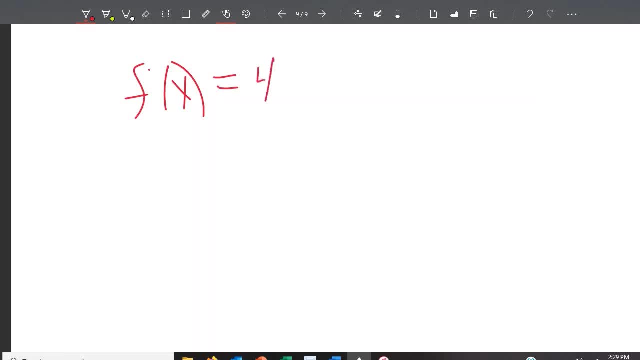 is well do. for x squared, I mean 4x cube, 7x squared plus 3x plus. oh, let's do 15. okay, so we, we would take all the factors of 15, the bottom, I mean the last number in the top and in. 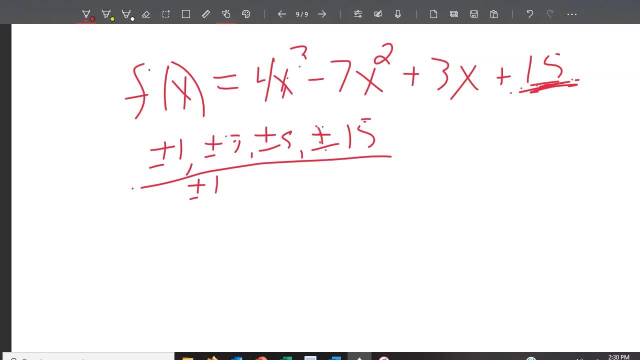 the bottom, we would put all the factors of four. Now, first thing I'm going to do is divide the top numbers by one. Now, divide the top numbers by one. we'll get plus or minus one, plus or minus three, plus or minus five, plus or minus 15.. I'm going to take the top and divide everything by two, So we'll 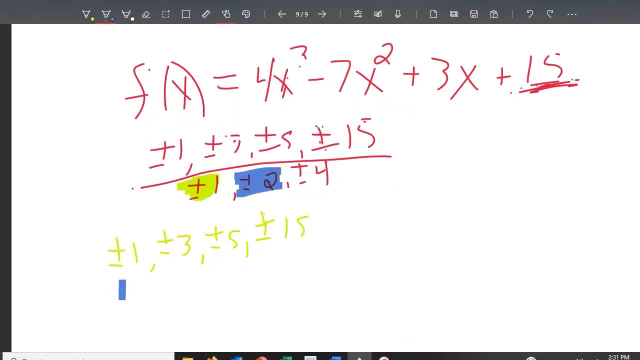 have plus or minus one half, plus or minus three halves, plus or minus 5 halves, plus or minus 15 halves. Then I'm going to take the fourth and divide it into everything in the top, So we'll have plus or minus 1 fourth. plus or minus 3 fourths plus. 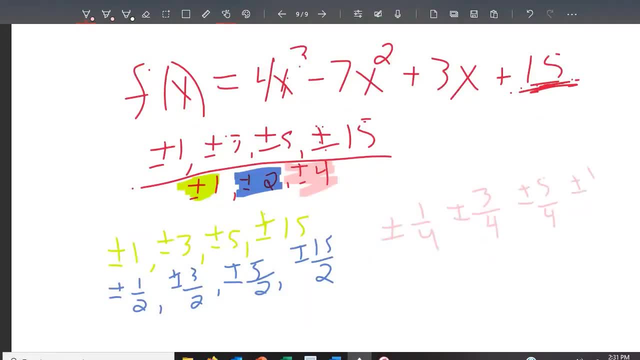 or minus 5 fourths. plus or minus 15 fourths. Now this is an extreme problem. There are 24 possible roots. Our goal is to use synthetic division and these numbers and try to find one that gives me zero at the end. This is where it gets very tedious. You have to take each one separate. You don't know. 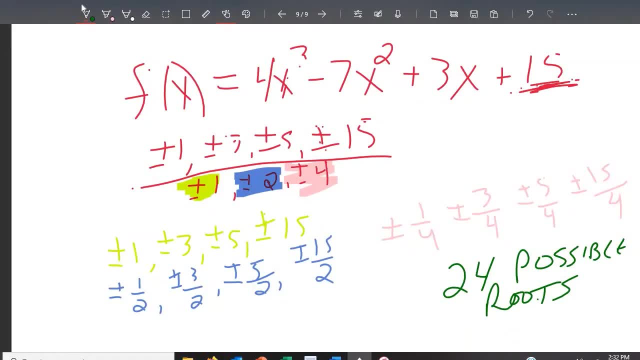 which one's going to work. You have to do them separate until you find a zero. Now, I would not have one this extreme on the quiz, but I'm going to do it, I'm going to do it, I'm going to do it. 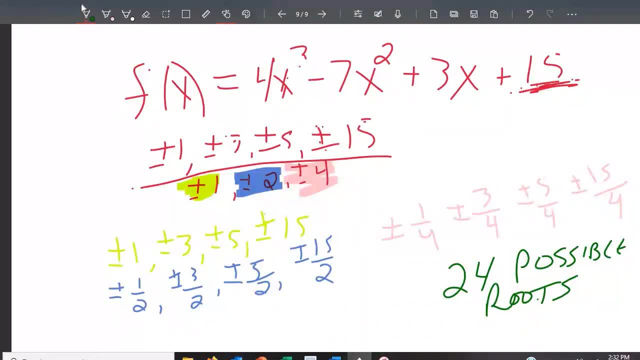 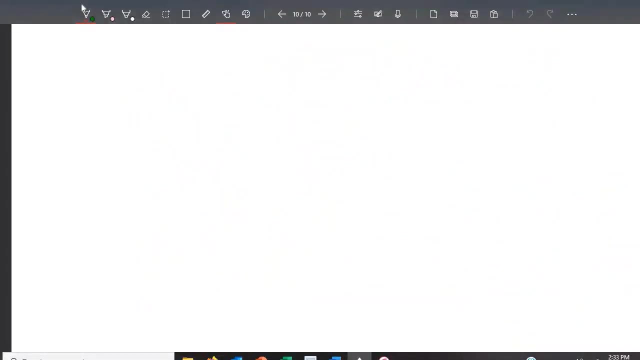 I do want to show you how you go about this. Let's do try to find a good one here. Let's start with. so I want to solve x cubed minus 2x squared plus 7x minus 4.. I already did this one earlier: Minus 4 equals 0.. Alright, first thing you do is list out your possible roots. 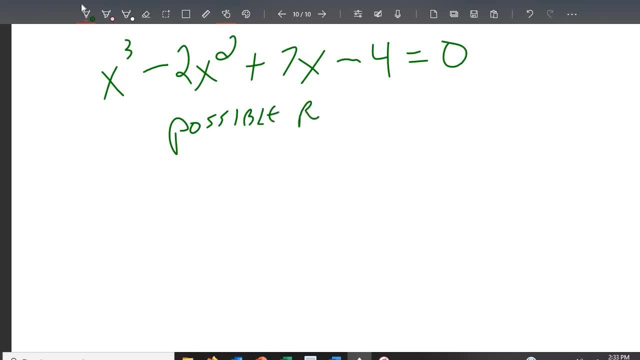 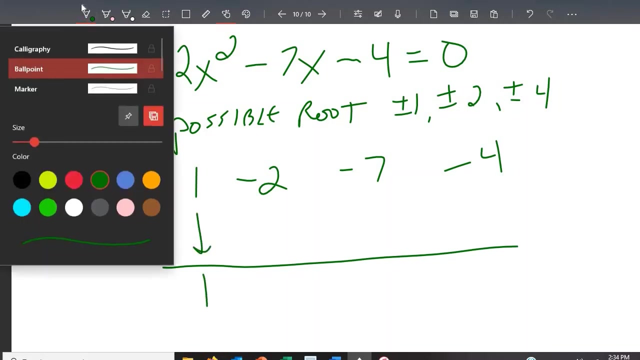 And I did this one earlier. The possible roots are plus or minus 1,, plus or minus 2,, plus or minus 4.. And you set up your synthetic division: Whoops, that should be a minus 7.. And that should be a minus 4.. And you set it up just like normal. But this time I don't know. 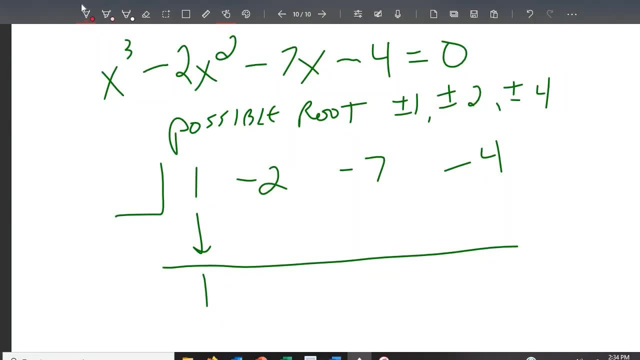 which number works. so we have to go check them, Literally check them. So I'm going to start with positive 1.. 1 times 1 is 1. Combine that together we'll get negative 1.. Negative 1 times 1 is: 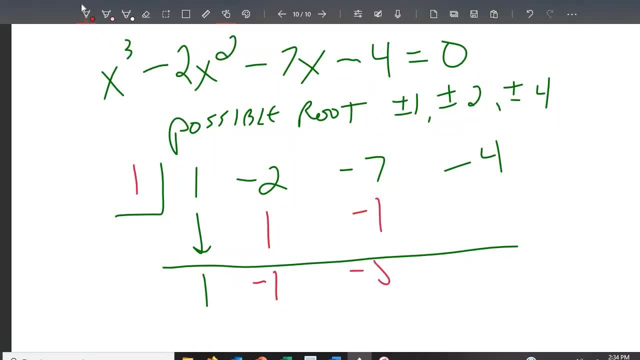 negative 1. Combine that together, we'll get negative 8.. Negative 8 times 1 is negative 8. And I get negative 12. Well, I need a 0 right there where that negative 12 is. So what that means. this positive 1 doesn't work. 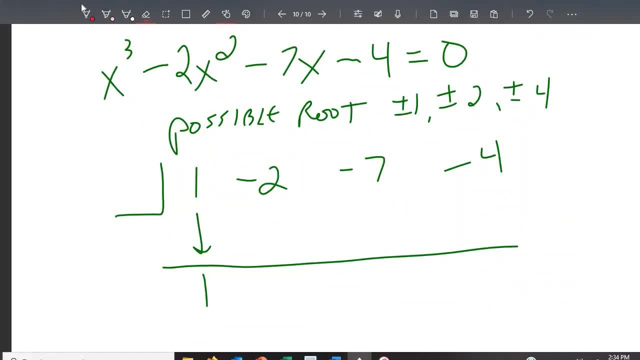 So then I choose another number out of that list, So I usually just start with 1.. 1 times 1 is 1., And I get negative 12.. Well, I need a 0 right there where that negative 12 is. So what that means. this positive 1 doesn't work. 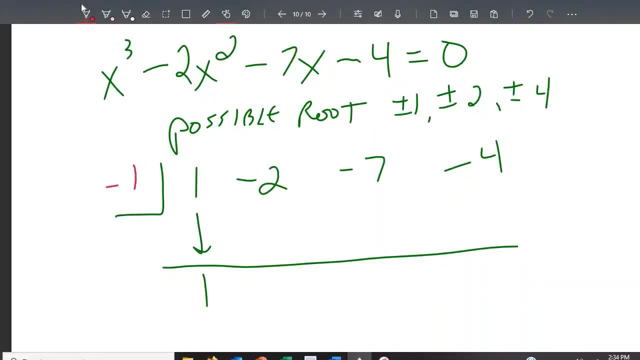 So let's start with 1 and work my way down. Let's try negative 1.. Well, 1 times negative, 1 is negative 1. That gives me negative. 3. Negative 3 times negative: 1 is positive 3. I get negative 4.. 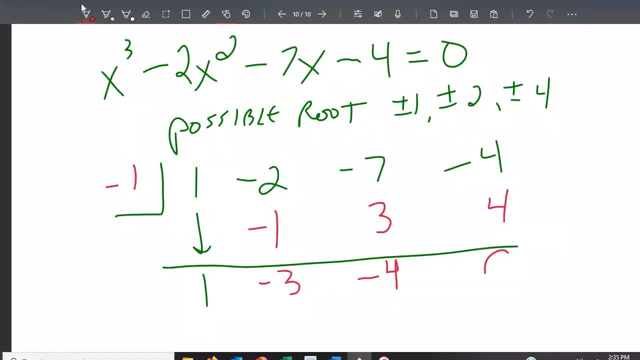 Negative 1 times negative 4 is positive 4.. And guess what I get: 0.. What that mean: This is a root. What that means: this is a root, which is the same thing as a 0, which is the same thing as my solution. So, one of. 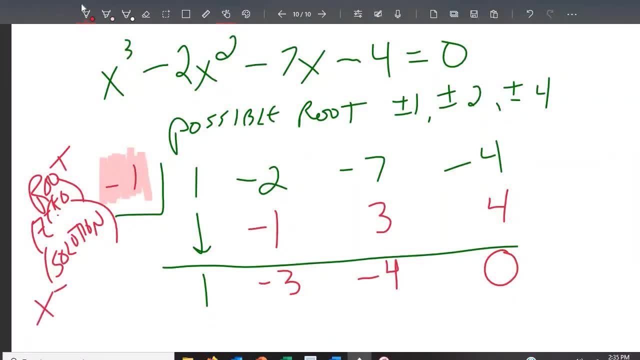 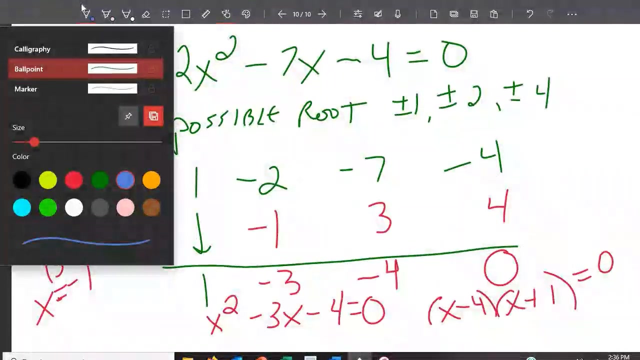 my answers for this problem is: x will be negative. 1. Put the variables back with the numbers and go factor that binomial, I mean factor that trinomial. it'll be x minus 4, x plus 1 equals 0. Now you know, we already know how to do this. This is: 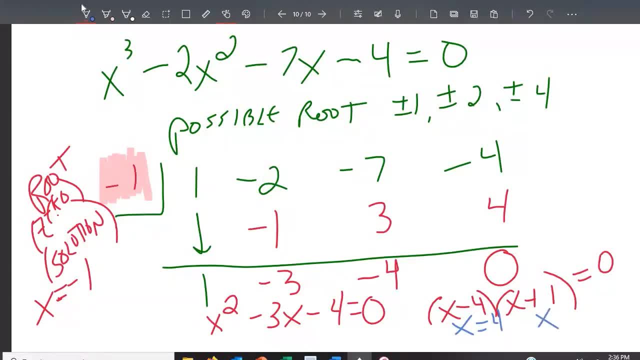 going to be a x equals 4, and this is going to be x equals negative 1.. Well, I've already got negative 1, so my other answer is x equals 4.. So that's one of my answers. I already had the negative 1, so this one has two answers. 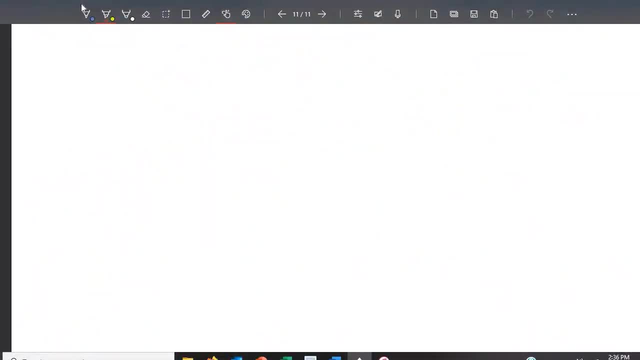 All right, let's do. we'll just keep on doing this. Let's do: 6x cubed plus 25x squared minus 24x plus 5 equals 0.. Okay, now here comes the possible. you know you've got to list out your possible roots. 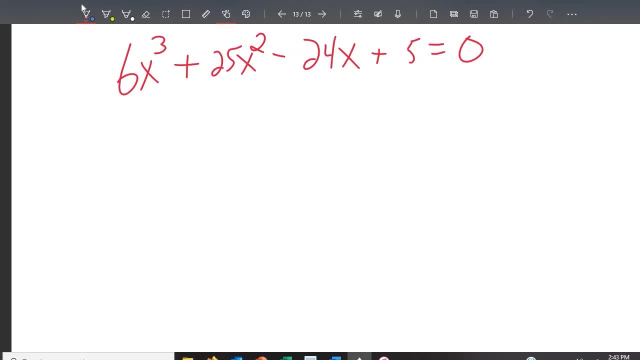 There's a question on the final, where it just says list the possible Possible roots. So remember it's always the last number, so it's the factors of the last number divided by all the factors of the first number. Okay, so we take every number in the top, divide it by 1, and we get that. 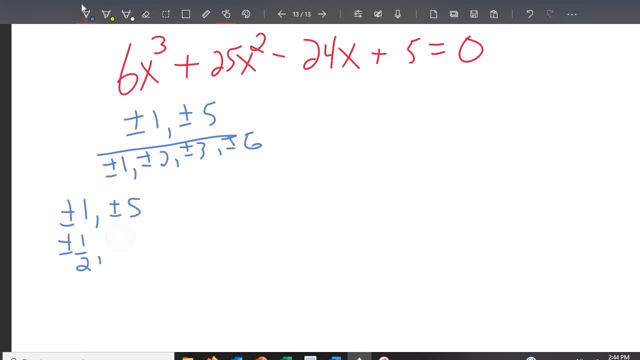 Take every number in the top, Divide it by 2.. Take every number in the top and divide it by 3.. Take every number in the top and divide it by 6.. Wow, what a mess. What a mess. 16 possible roots and only 4 of them are whole numbers. 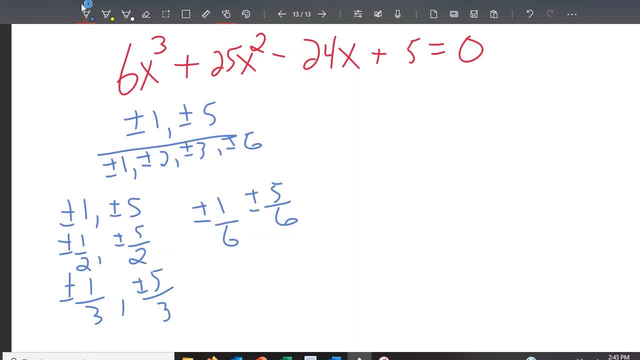 Let's hope there's a whole number that works, because I don't want to deal with these fractions, But let's just go do the synthetic, see if we can find one that works. I always try to do the whole numbers first and then, if I have to, I'll do the fractions. 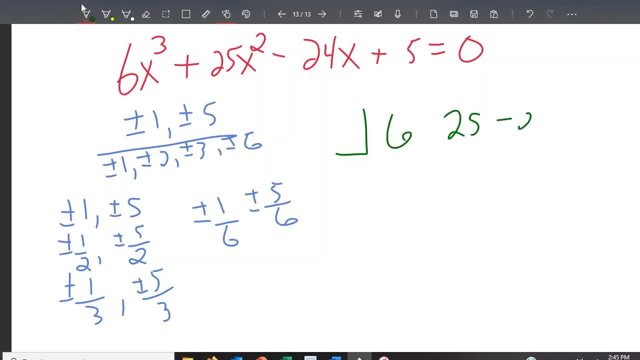 So I'm going to definitely start with the whole numbers. Okay, All right, All right, Let's just start with 1.. Again, All right. 6 times 1 is 6. Combine that, we'll get 31.. 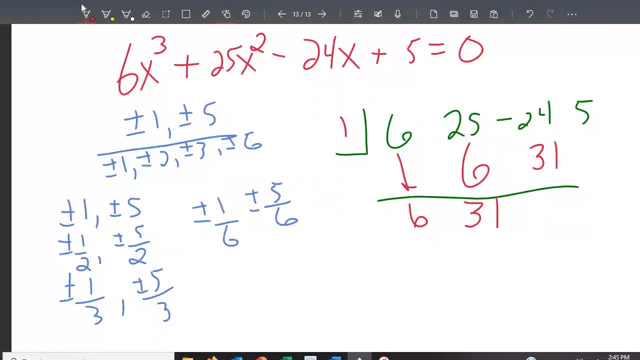 31 times 1 is 31.. I'll get 7.. And that's definitely not going to give me a 0. So start over. Let's try negative 1.. 6 times negative 1 is negative 6.. That's going to give me 19.. 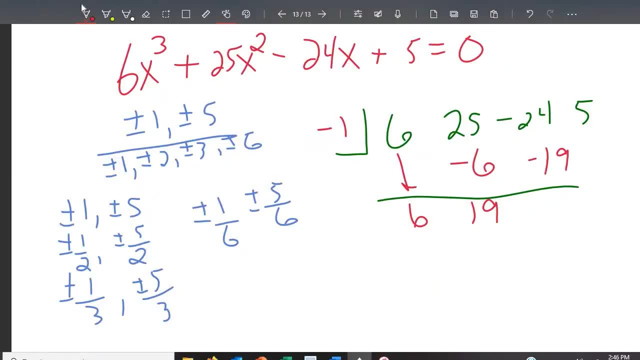 19 times negative. 1 is negative 19. And that's not going to work. This is the way it works sometimes. You just have to check 3,, 4,, 5 of them. You know, Let's try 5.. 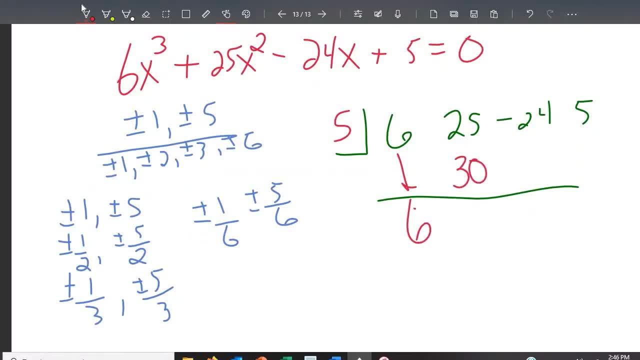 6 times 5 is 30.. 6 times 5 is 30.. That gives me 55.. I hope you can tell that ain't going to work, So let's try negative 5.. I sure don't want to have to do a fraction. 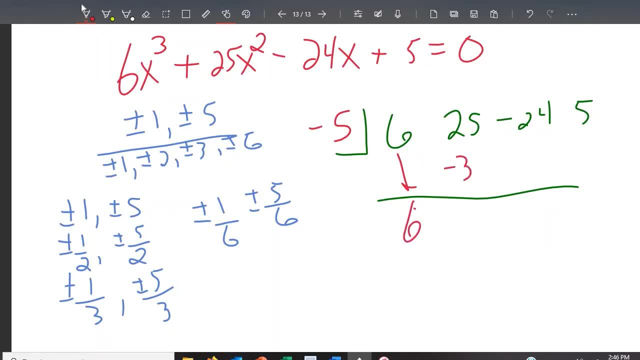 6 times negative 5 is negative 30.. That gives me negative 5.. Negative 5 times negative 5 is 25.. That gives me 1.. 1 times negative 5 is negative 5.. And I get 0..